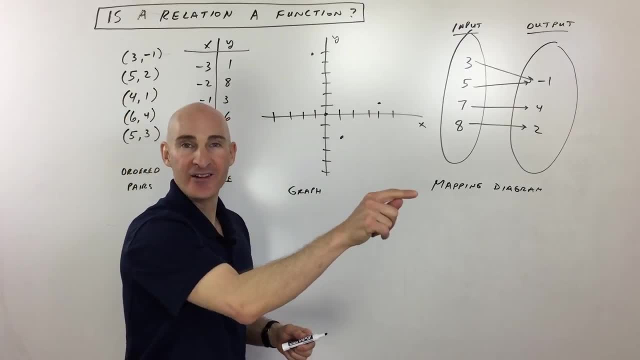 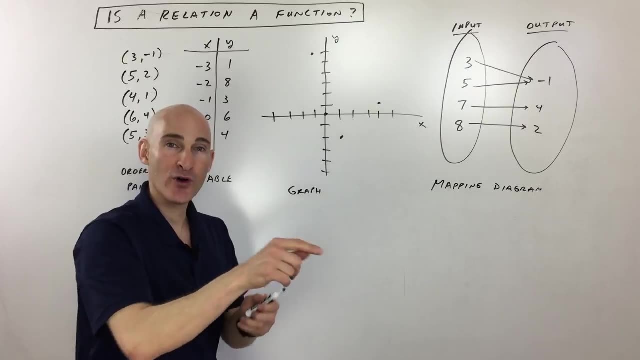 vending machine. Like if you go to a vending machine and you push A1, right, and one time you get a Coca-Cola and one time you get a Pepsi- okay, that's unpredictable. You have one input but you're actually getting more than one output. You don't know what you're. 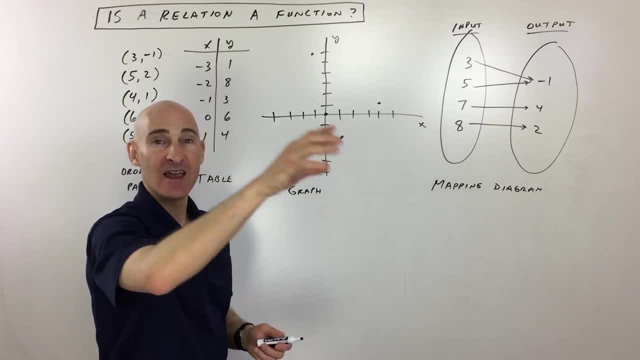 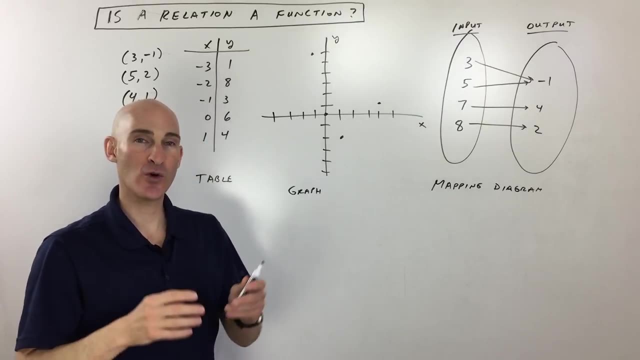 going to get right Now. it's okay to press A1 and get a Coke and press A5 and get a Coke, because when you press that button you know what you're going to get. So it's okay to have more than one input going to the same output. Okay, I'll show you in these examples. 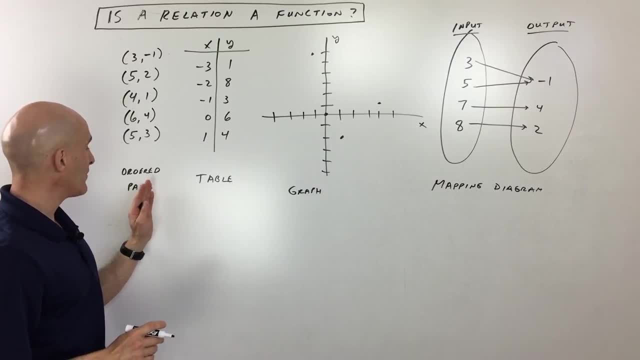 what I mean. So, first of all, we can display these relations as ordered pairs, tables, graphs, mapping diagrams et cetera. So with the ordered pair, you can display the relations as ordered pairs, tables, graphs, and you can see that we're pairing the X value with the Y value, X with Y, X with Y. 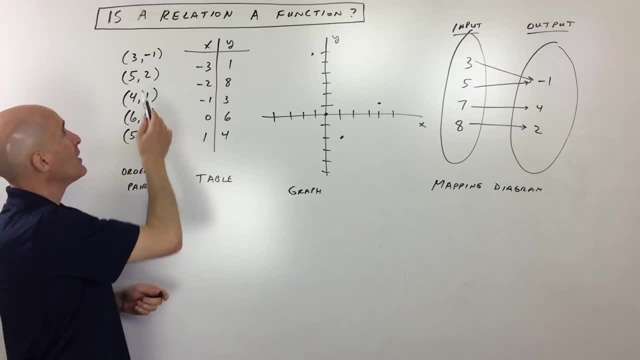 X with Y and so on. What we want to be careful of is: you don't want to have the same input going to two different outputs like that, right, And that's what's happening here. You can see 5 is mapping to 2, but 5 is also mapping to 3.. Back to that vending diagram. we're 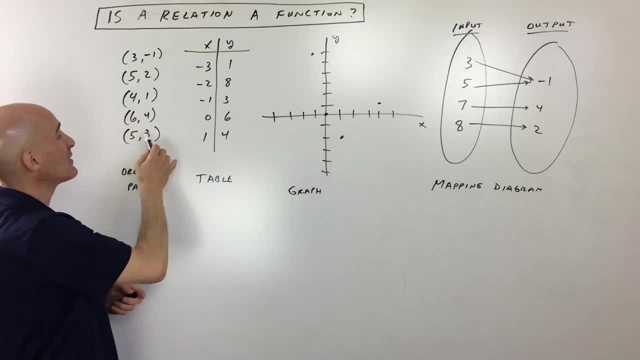 pressing the button 5.. One time we get 2 as an output, one time we get 3.. So this one is not a function. So I'm just going to write: not a function. okay, For the second one, this table same thing. You're matching an X value with a Y value. 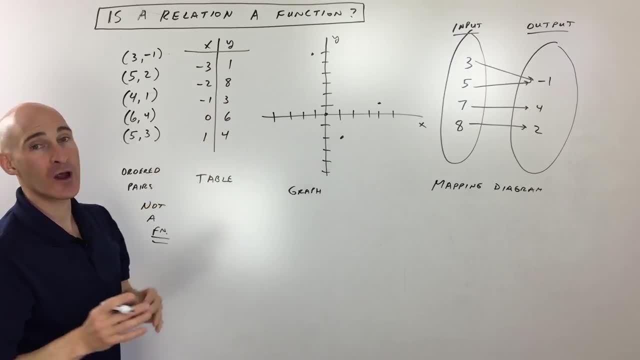 Negative 2 maps with 8, negative 1 maps to 3, 0 to 6, 1 to 4.. What you're looking for is a repeated input, a repeated X value, So you can see the X values are not repeated. 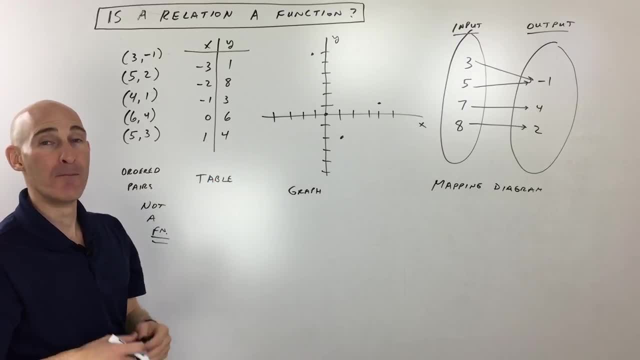 so we're not in danger of having one input going to multiple outputs. This one's okay. This one is actually a function, So I'm just going to say function Fn. This one, okay, is a graph And again, you know, a graph is really just like a plotting of X. 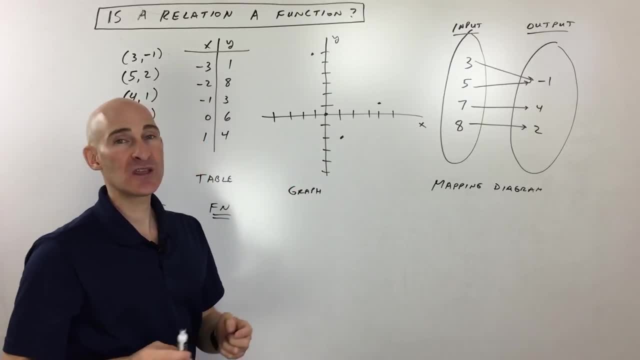 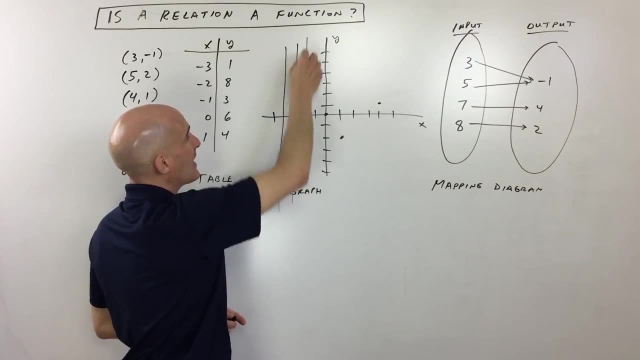 coordinates and Y coordinates okay, for each individual point. Now, when you're looking at a graph, a nice way to check to see if it's a function is to do something called the vertical line test. What you do is you draw a bunch of these vertical lines and 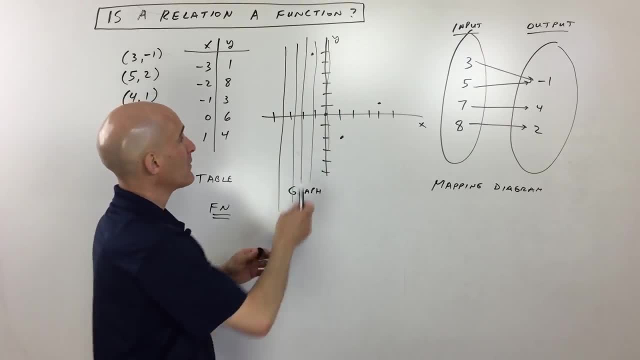 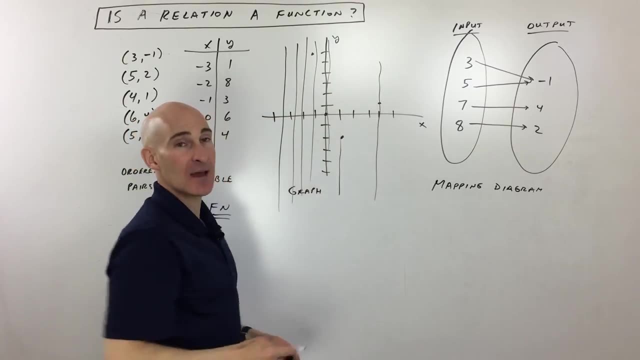 what you're doing is you're seeing if it crosses more than one point for a given vertical line. Now when you scan across here, you can see that's never the case. Every time you know I draw a vertical line, it's only crossing at most one point, Whereas if I put another. 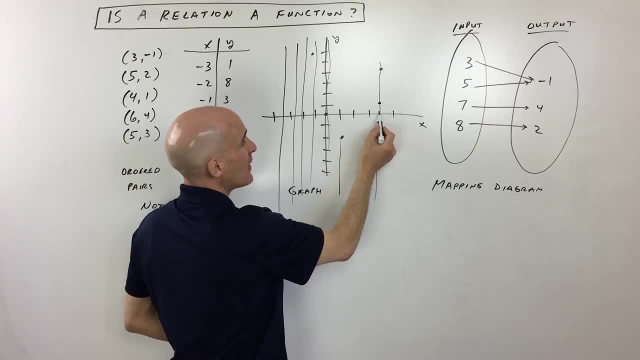 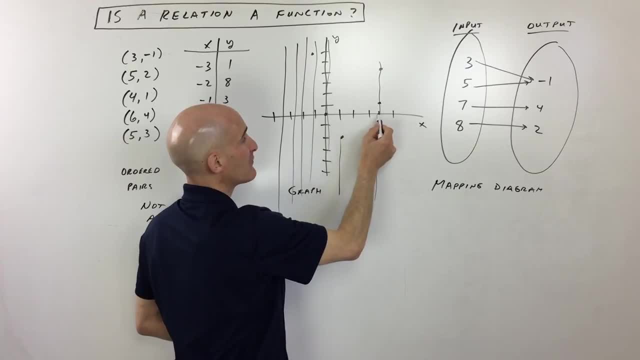 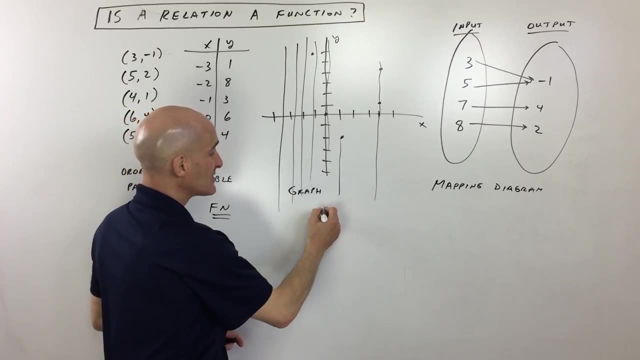 And I'm going to do a vertical line test And I'm getting a Y value of 1. And I'm getting a Y value of 4.. So for that particular input, that X value, I'm getting more than one Y value. So as it stands now it fails that vertical line test. It means that it's not. 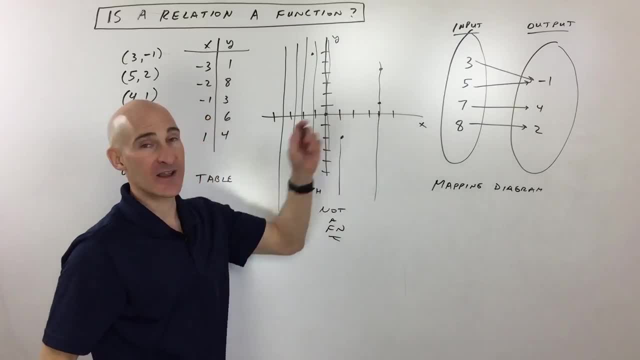 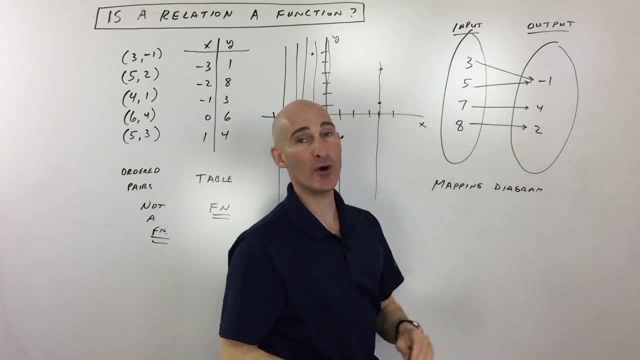 a function. Okay, All right, so that's that one. And then mapping diagram: just like it looks like you have an input and output and you're mapping or drawing an arrow from the input to the output. Now some students make a little mistake with the mapping diagram. 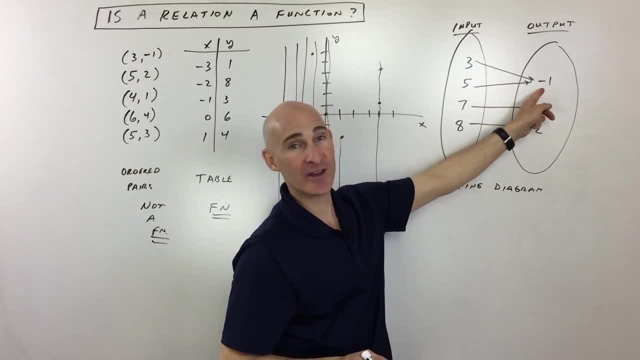 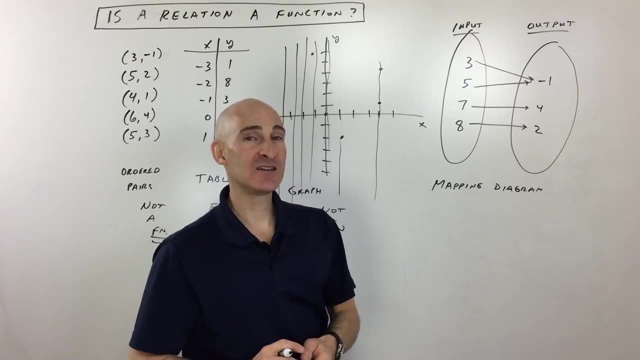 because they see these arrows going to the same output like that And they say: wait a second, something doesn't look right here. 3 goes to negative 1,, 5 goes to negative 1.. But again, if we go back to my vending machine example, if you push the button 3, do you know what you're? 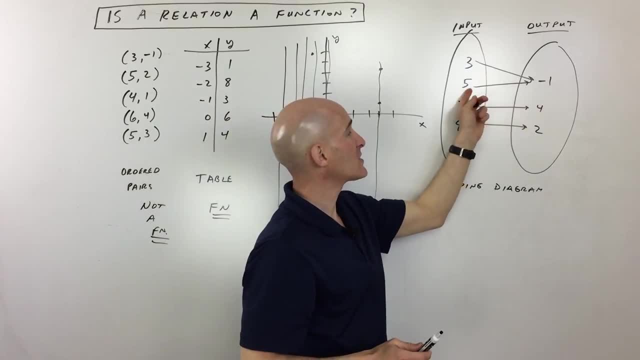 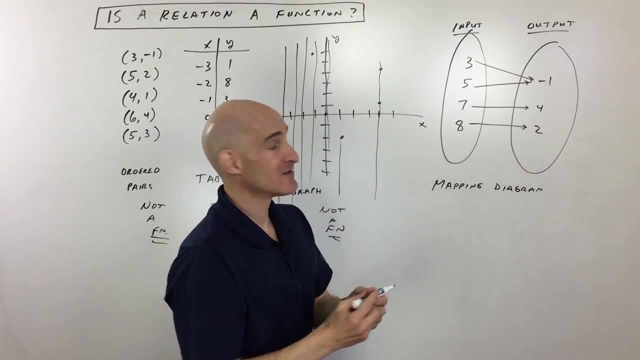 going to get for your output? Yes, you know you're going to get negative 1.. If you press 5, do you know what you're going to get? Yes, negative 1.. That's okay, That's predictable. That's a function. What you don't want, and I'm going to change the setup of this particular one- 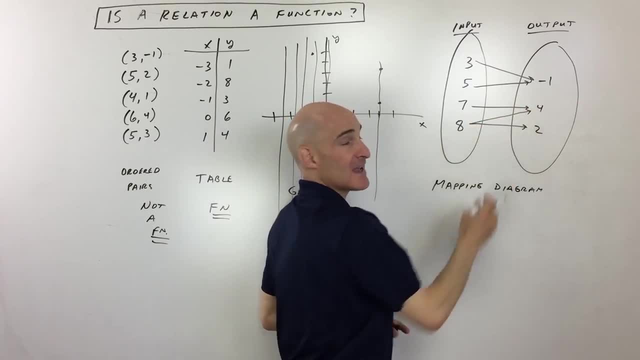 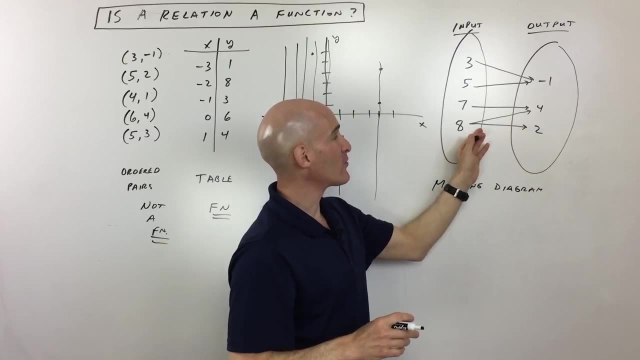 is you don't want 8,, for example, going to 4 and 8 going to 2.. So you press that button on the vending machine. One time you get 4, that comes out whatever that represents Coca-Cola. or you press 8 and out comes Pepsi. 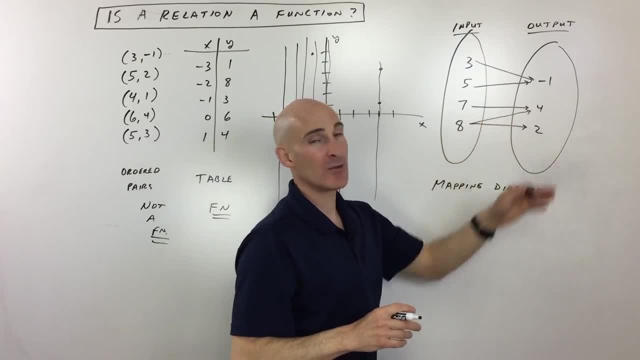 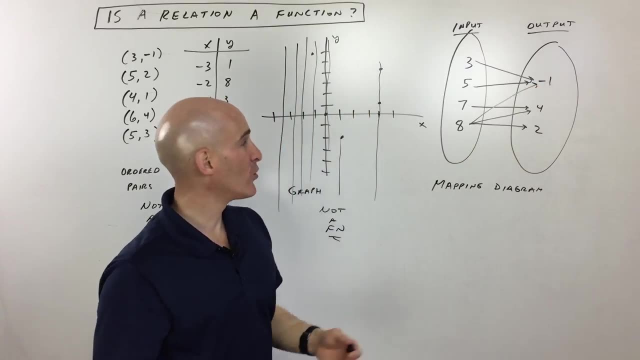 right. So you don't know what your outcome is going to be. Here you have one input going to more than one output. It doesn't just have to be 2.. You can have 8 also going to negative: 1,, 4, and 2.. We don't know what the output's going to be. We don't know what the end result's going. 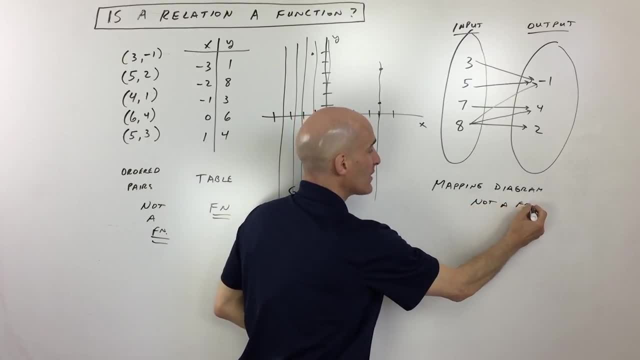 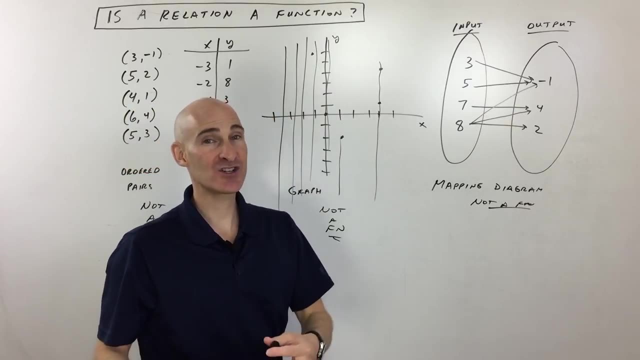 to be. So this one is not a function. So basically, a relation, like we said, is a pairing of inputs with outputs, But you want to make sure that not every relation is a function unless it satisfies each input just goes to one output. So I hope this helped you understand how to work with. 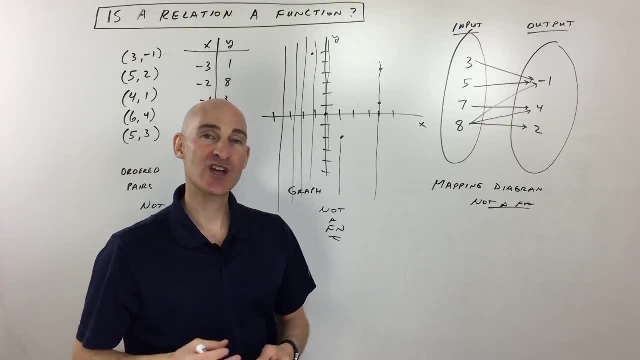 relations and functions better. Subscribe to the channel. Check out tons more math tutoring videos on my YouTube channel, Mario's Math Tutoring, And if you have suggestions or you have something that you want me to do a video about in the future, I'll definitely consider it if it's.